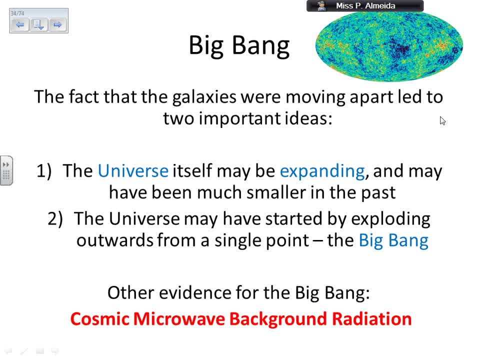 So this comes from the observations of the redshift? okay, So the fact that the galaxies were moving apart led to two important ideas. One is that the universe expanded- The universe itself may be expanding and they have been much smaller in the past- and the other was that the universe may have started by exploding or rapid expansion outwards from a single, very hot and dense point, and we call this the Big Bang. 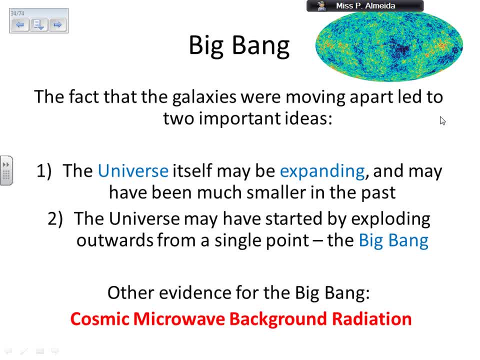 Now, as everything in science, you try to give an explanation to the observations that you have, and the Big Bang was not the only theory about the observations that we had about redshift. There was another theory, quite famous, that is called the steady state theory. that said that the redshift observations were happening because the universe had white holes and the white holes would do the opposite of black holes. 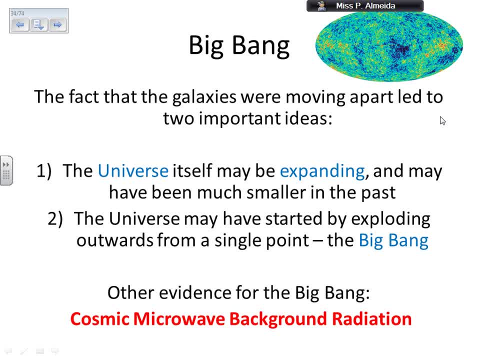 So the white holes would eject material to the universe. So you would have a steady state universe, meaning no beginning and no end. it was always there, just the way that it looks. So you would have a steady state universe, meaning no beginning and no end. it was always there, just the way that it looks. 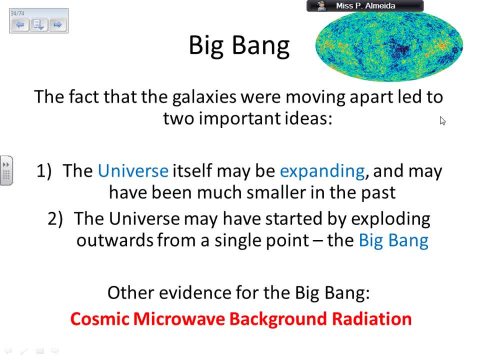 like now, however, things were moving apart, because there were these white holes that would appear out of nowhere everywhere and they would create space, because they would put matter into that universe. okay, now redshift was showing that things were moving away from each other. so the redshift- 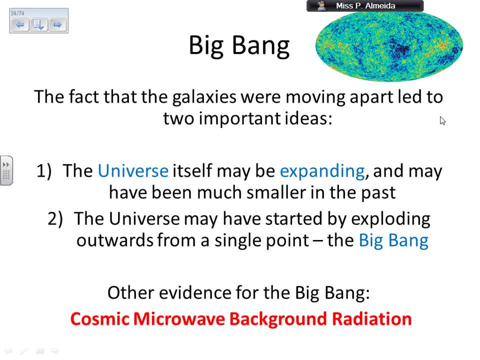 could be explained using the big bang theory or the steady state theory. so what scientists need to do is go and look for more evidence right to try to prove that their theory is correct, and the other evidence that came for the big bang and that made it win against the steady state. 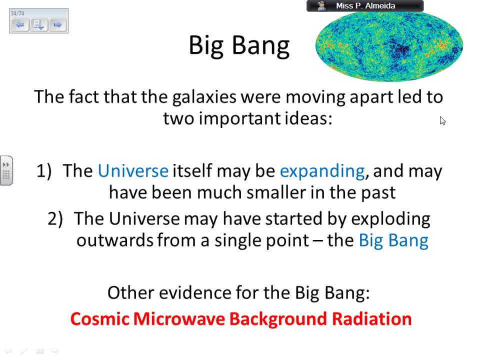 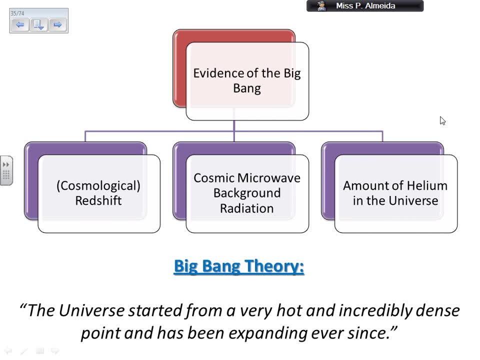 theory is this one called the cosmic microwave background radiation. okay, now, um, so the big bang ended up by winning. let me just tell you that there is another evidence for the big bang, which is the amount of helium in the universe, and they will all be explained in the next slide, okay. 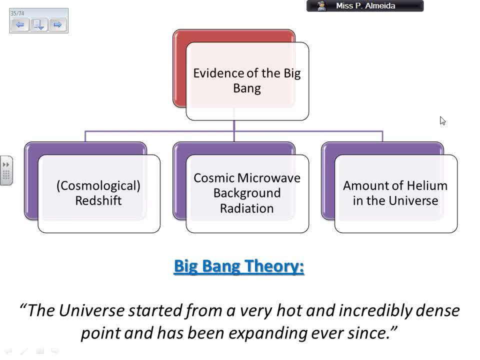 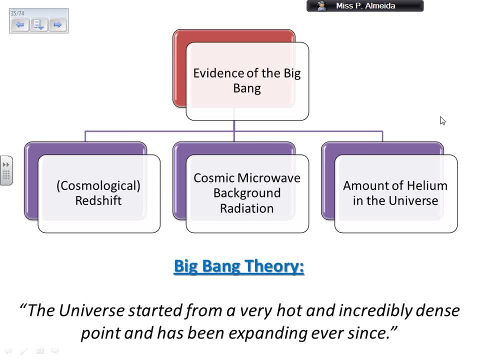 dense point and has been expanding ever since, is number one, the redshift, the cosmological redshift. okay, so it's not the redshift of having an ambulance passing by, it's a cosmological one. so, from the cosmos, what we see around, uh, us, in terms of the universe, okay, galaxies moving away from each other. okay then the cosmic. 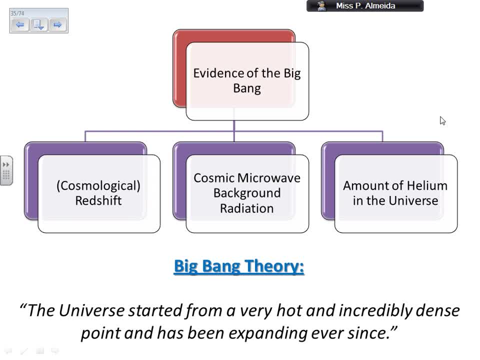 microwave background radiation, that i'm going to tell you a little bit about it, and then the amount of helium in the universe. okay, so these are the three evidence- uh, that are the three types of evidence that we have- that um makes us believe at the moment that the big bang is the best theory. 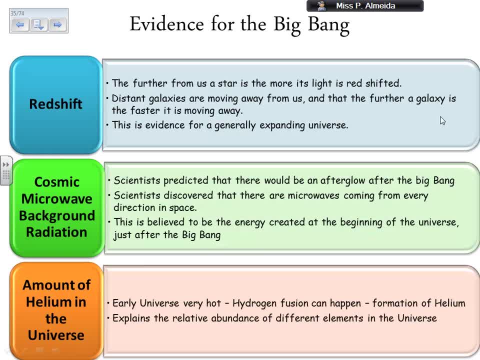 to explain how the universe may have started and how it's going to change, the way the universe is able to work and what kind of tech they're going to be able to have to deal with. we're going to have to it. okay, so the explanation of all of these, or summary about all of these, the 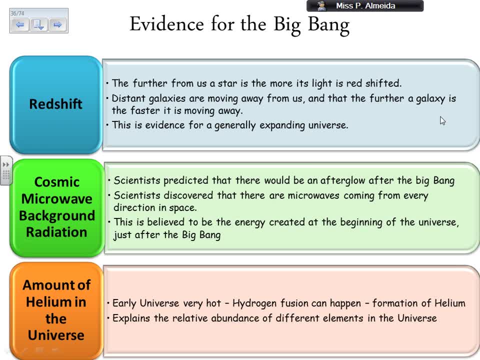 redshift. the further from us a star from out, for the further from us a star is. oh sorry, you know, because I know what is written on the slides, but I have, or I have, an idea, but sometimes I want to read it to make sure that I'm not you. 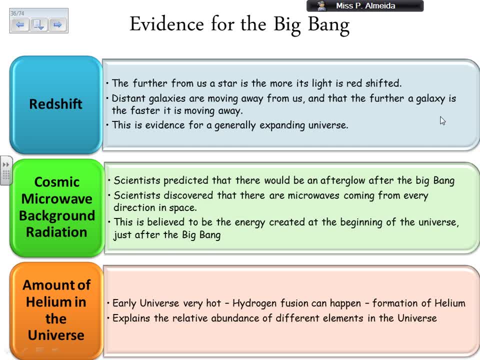 know missing out something and then these things happen. so the further away galaxies from us, the more the light is redshifted. okay, distant galaxies are moving away from us, and the further away the galaxy is, the faster is moving away from us. so this is an evidence for generally expanding universe. this was 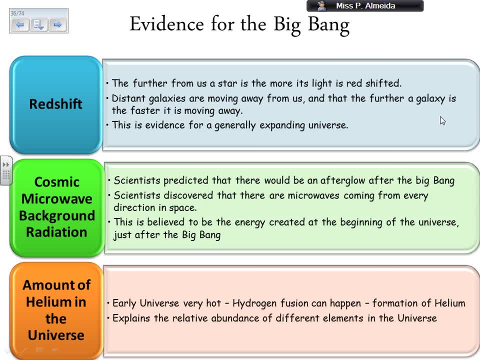 evidence for the Big Bang. this was also evidence for the steady-state theory, now cosmic microwave background radiation, which this is not going to be the only video that I'll do about it, by the way. the scientists predicted that there would have been an afterglow after the Big Bang. 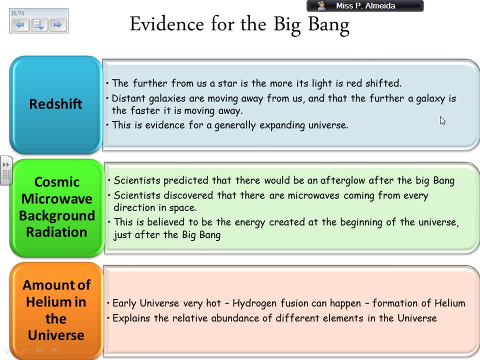 so if this happened, then we should have had this cosmic microwave background radiation to form, and if I'm not wrong, this was formed ten to the power of minus four seconds after the universe, or after the Big Bang. okay, so the scientists did discover that they were microwaves coming from every direction in space and 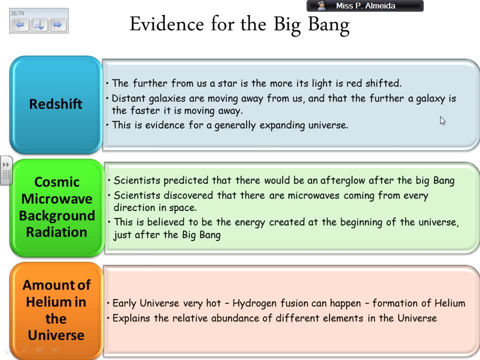 this is to believe to be the energy created at the beginning of the universe just after the Big Bang, so about ten to the power of minus four seconds after. okay, now this microwaves. I'll tell you a little bit more about them, but when the scientists were predicting it, they did predict that, whichever radiation it would. 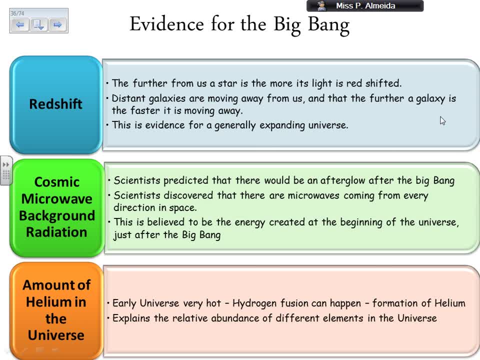 be would be in the microwave region. so when you find something that just matches your theory, your calculations, your assumptions, then this is great. ok, so this was really the thing that made us believe that the Big Bang is the best theory at the moment to explain how this would happen. 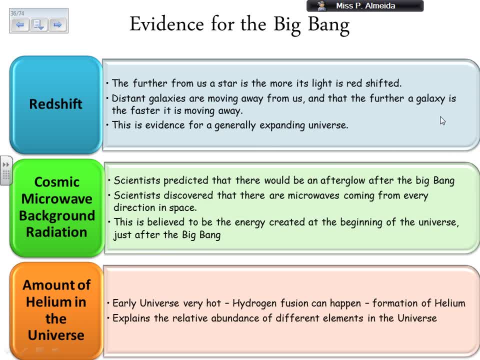 So, with this in mind, I'm going to go and talk about another theory, and this is where I'm going to talk about the Big Bang. the universe may have started, and this was worth the noble prize in, if i'm not wrong, 1967. okay. 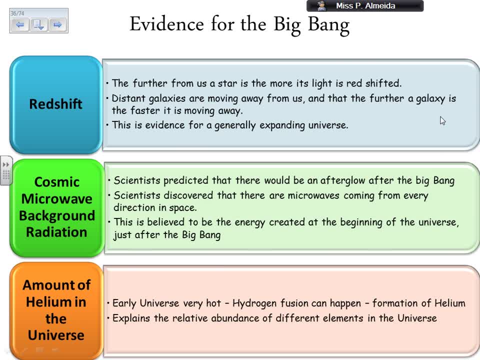 and then the other evidence for the big bang is the amount of helium in the universe. okay, so the early universe was very hot, so hydrogen could fuse, could fuse into helium and form helium. okay again, go on a video about stars. um, i believe is in my other playlist called classification of 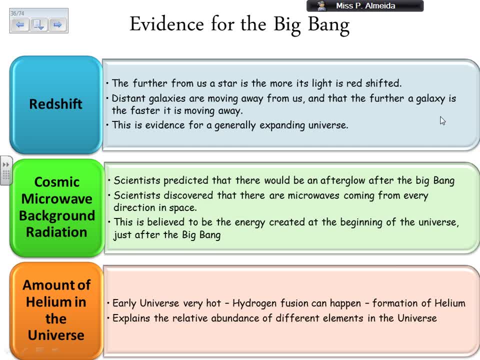 stars, where i have the explanation about fusion. okay, now this amount of helium in the universe. it does explain the relative abundance of different elements in the universe. so, because the universe would be very hot, i could have hydrogen fueling, uh, fusing into helium and then other structures making further fusion. okay, like for example, stars and the relative abundance of 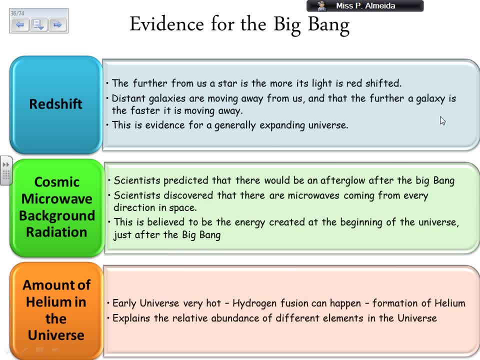 different elements in the universe, where hydrogen and helium make about 19 percent, but all the rest is there as well. the other two percent, or about two percent, is there as well and it does much on our observations on how they were formed. it does much for evidence for a very hot, early universe, okay. so 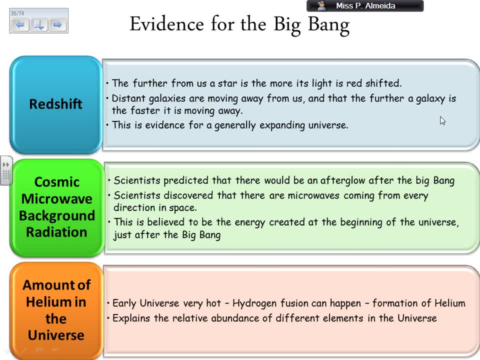 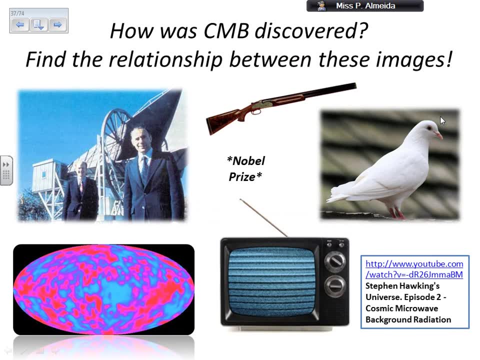 all of these three are evidence for the universe starting with a Big Bang. okay, now this cosmic microwave background radiation. the story on how it was discovered was quite interesting, actually quite funny in a way. beats out for the pigeons, but um, I did have here a video. feel free to search for this video. 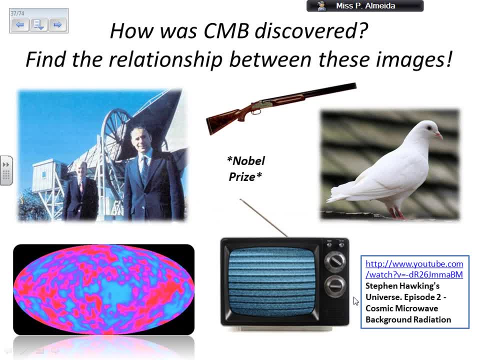 I tried the link and the link is not working at the moment. I tried putting the searching from the video for the videos name alone. I couldn't get it to work either, but feel free to look for it. but basically what happened was scientists were looking for these microwaves coming everywhere from. 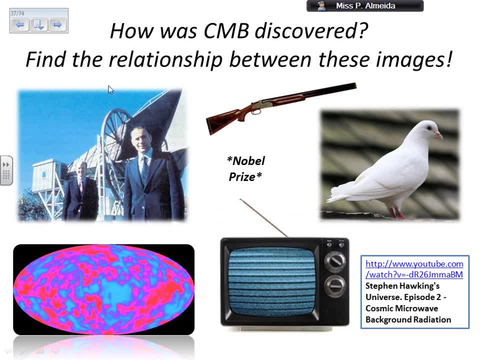 somewhere and they were looking for these microwaves coming everywhere from space and they had this type of equipment. okay, to look for this radiation at the same time. by coincidence, while one of the scientists was in a room with one of his friends, his friends did receive a phone call. 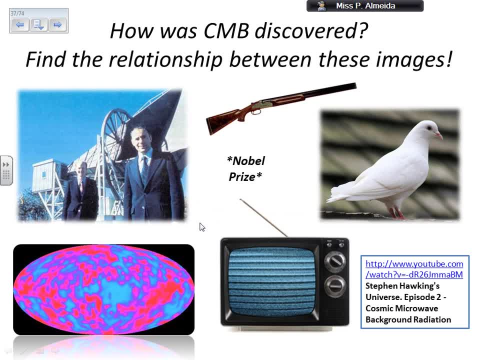 where another friend was kind of moaning to him. this other friend worked in a TV station and he was moaning to him that they had this noise, this annoying noise, this background noise that was coming from the radio station, and he was moaning to him that they had this noise, this annoying noise, this background. 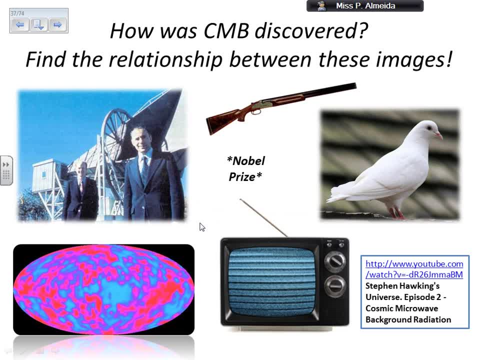 noise and they couldn't explain it. and it didn't matter where they would move: they were getting this noise. and this actually catch the eye, or actually the ears, of one, the scientist that was looking for the cosmic microwave background radiation, because it looked like they were finding something. that that's what they wanted to find. okay, that they were. 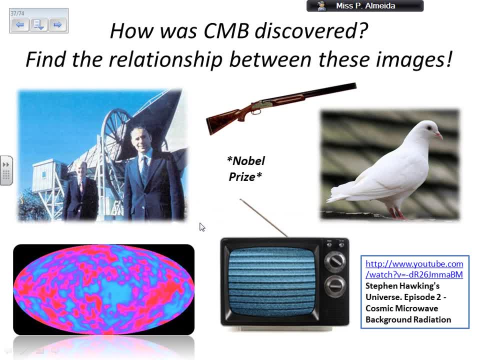 looking for as well. okay, so at first they thought that the reason for this interference, this annoying noise, was the noise in the background was the pigeons, because there were pigeons nearby the antenna. so they decided to um try to get the pigeons to move away. so they scared the pigeons out and then they cleared. 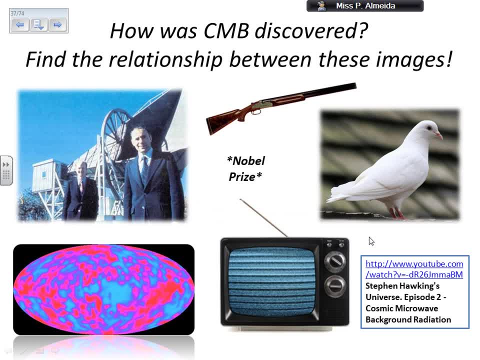 all the droppings and all these things and, um, this didn't work. and then the pigeons came back. so, unfortunately, um, they did kill the pigeons, okay, so they shot the pigeons and they're like: right now there is no more background noise. and guess what? there was still background noise. 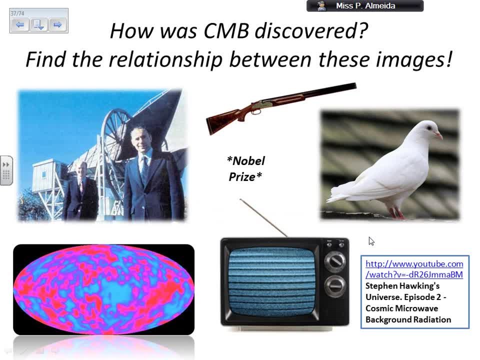 it was not the pigeons, creatures they were creating this. this was the cosmic, microwave background radiation that was coming everywhere from space. cosmic because it comes from space. microwave because that's the region in the electromagnetic spectrum where the radiation is from background, because it's always there, is always present. you cannot get rid of it.